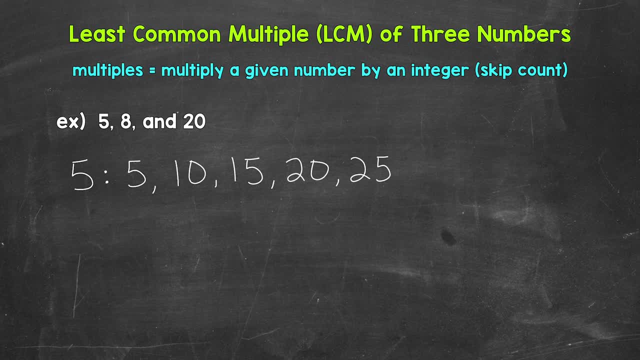 Now I stopped at 25 because multiples go on forever, They are endless, They are infinite. My suggestion is to list 4 or 5 multiples of each number when looking for the least common multiple. So let's start with 5.. So list 4 or 5 for each number. 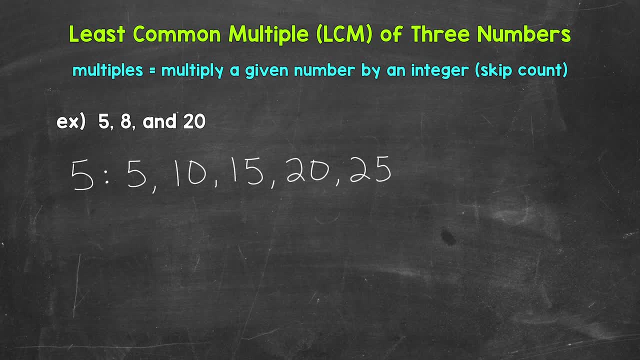 Look for any in common, specifically the least common multiple, And if you don't have any in common, you can always extend the multiples lists. Now let's list the first 5 multiples of 8.. 8 times 1 is 8.. 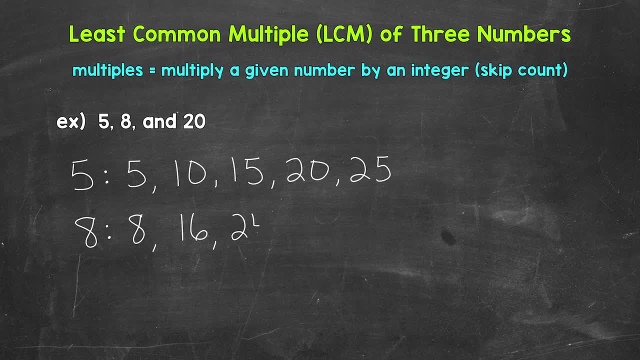 8 times 2 is 16.. 8 times 3 is 24.. 8 times 4 is 32.. 8 times 4 is 32.. And then 8 times 5 is 40. So 8,, 16,, 24,, 32,, 40,, so on and so forth. 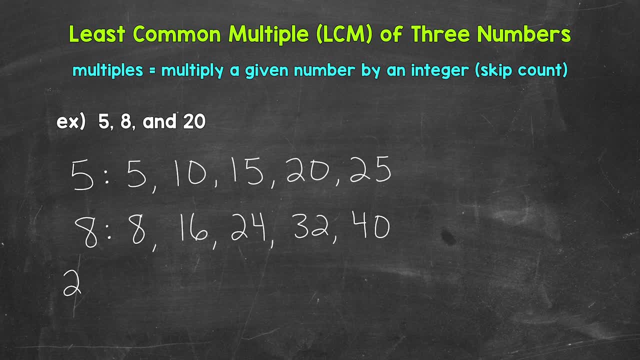 And then, lastly, let's list the first 5 multiples of 20.. So 20 times 1 is 20.. 20 times 2 is 40.. 20 times 3 is 60.. 20 times 4 is 80.. 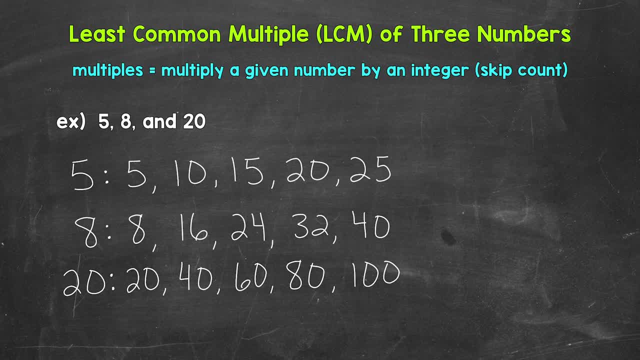 And then 20 times 5 is 100.. So 20,, 40,, 60,, 80,, 100, so on and so forth. Now that we have some multiples listed for each number, we can look for common multiples. 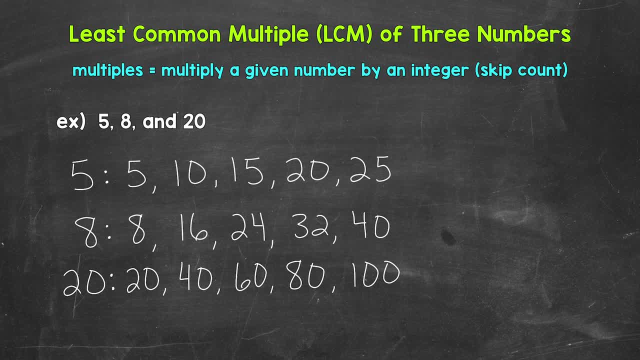 And specifically the least common multiple, So the smallest multiple in value that they all share. But as of right now, we do not have any multiples that all 3 of these numbers share, So we need to continue our lists Now. as far as 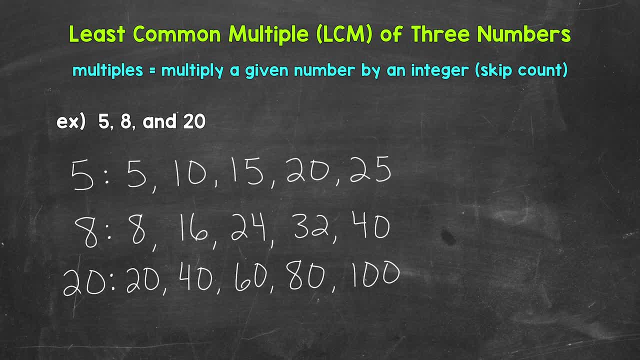 our lists of multiples. for the multiples of 20, we are at 100.. For the multiples of 8, we are at 40.. For the multiples of 5, we're only at 25.. So let's extend the list of multiples of 5.. 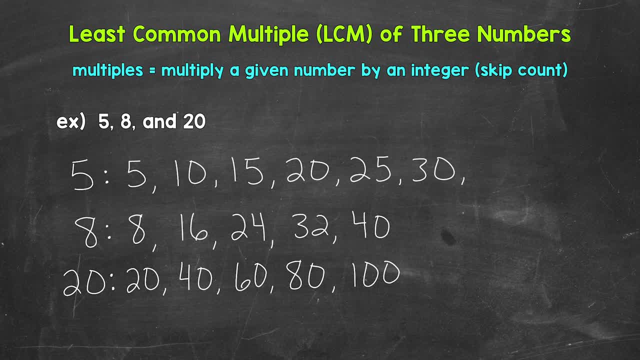 So after 25, we have 30,, then 35, and then 40. Now 40 is going to be a common multiple, A multiple that is not a common multiple, A multiple that all of our numbers share And, specifically, it's going to be the least common multiple.